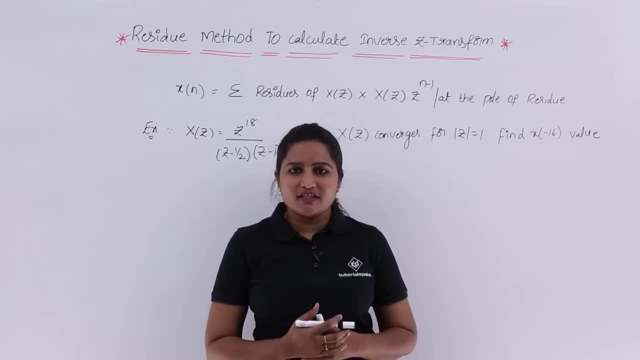 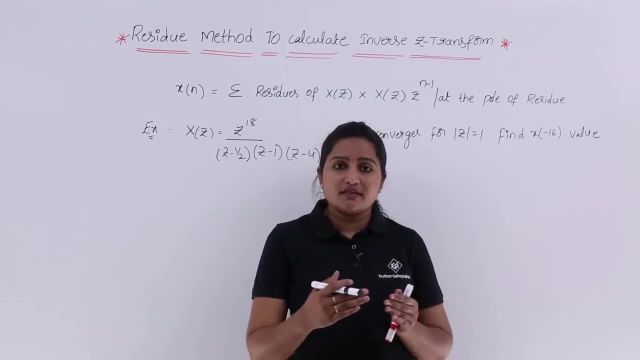 In this video we are going to discuss residue theorem to calculate inverse jet transform. Up to now we discussed three methods: general method and long division method and partial fraction method. General method: we done so many problems on that- how to decode the samples from the given. 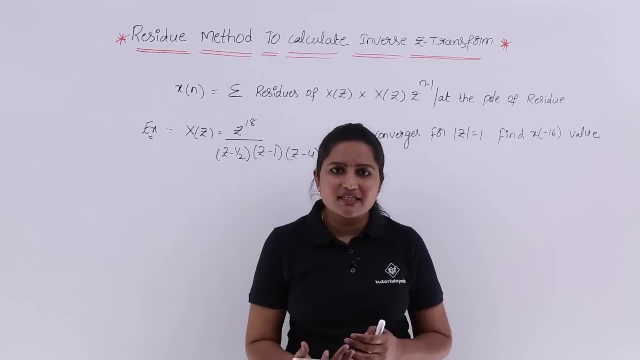 equation of jet transform and after that, if rational jet transform is given, long division method or partial fraction method we can use, and here one more method is there. So this method will specially use when they are asking the value of the jet transform at any instant of time. 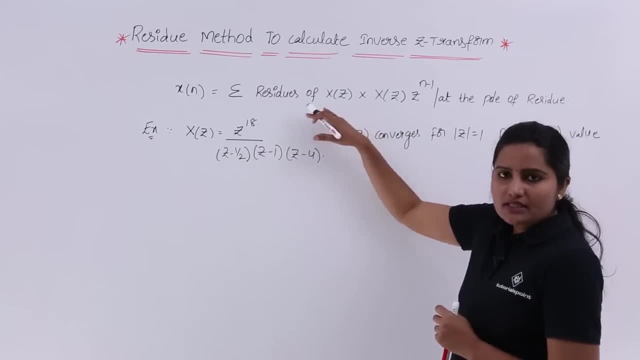 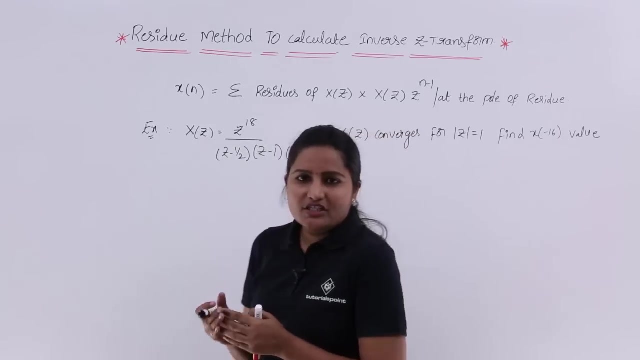 So here this is residue theorem. this is the equation for residue theorem. x of n is equivalent to summation of residues of x of z into x of z into z, power n minus 1 at the pole of residue. So this equation may not be understood. now if we consider one example, then it is very clear. 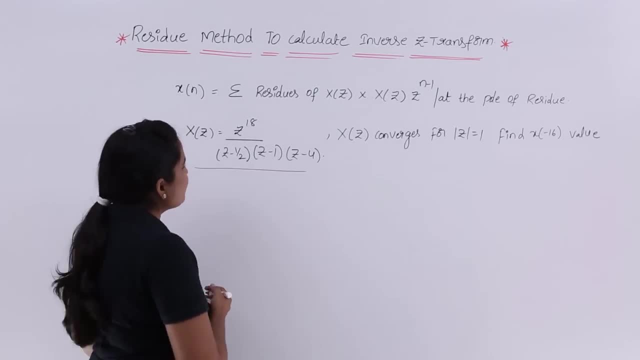 So here I consider this example: x of z is equivalent to z power 18 divided by z minus 1, by 2, z minus 1, z minus 4.. So here this is our jet transform of any signal, x of n. Now we need to consider the inverse jet transform. find the x of minus 16 value. that means: 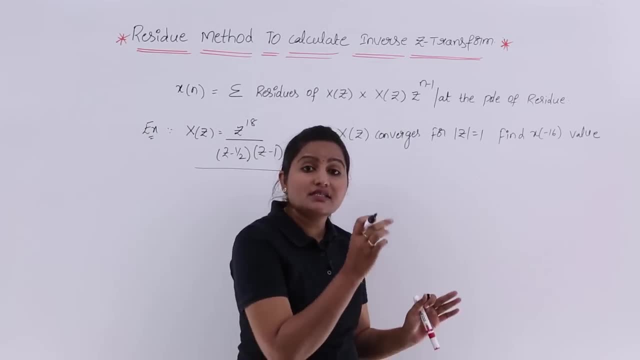 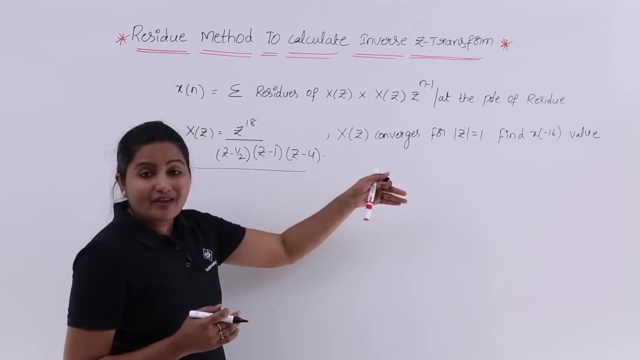 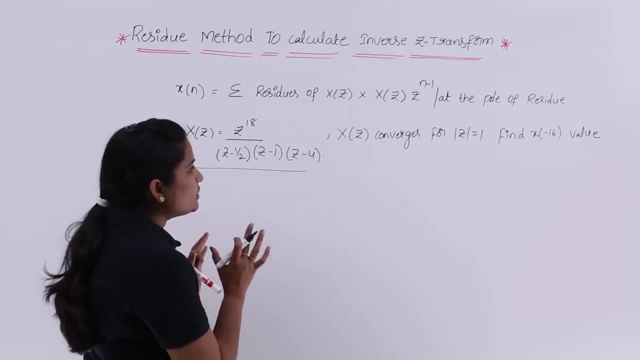 there are not asking x of n, X of n. at some instant of n is equivalent to minus 16. they are asking So in that type of cases. so if any value they are asking, if they are asking any particular value of the signal, then you can go for this method. So here, residues are nothing but whatever. 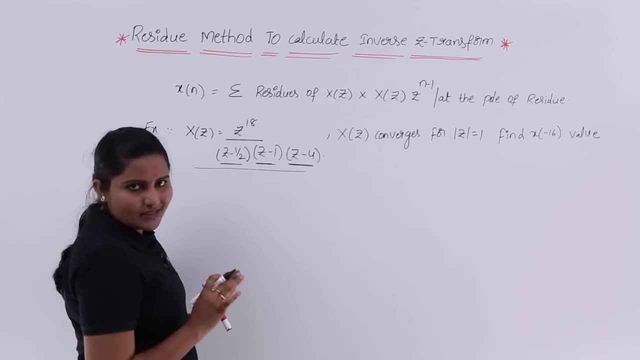 the denominator groups are there. those are called as residues. So here I am using residue theorem directly directly to write inverse property of n. Similarly, for a nail Hit poor's forces, I am removing n from 1, this 0. Now I am taking n equal to 0 and it gives me a value instead, the value of z. that is Goodness. 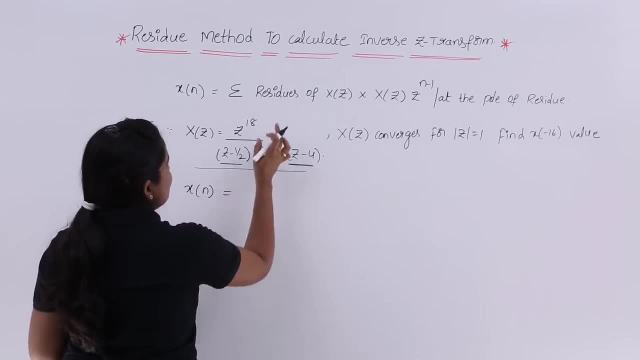 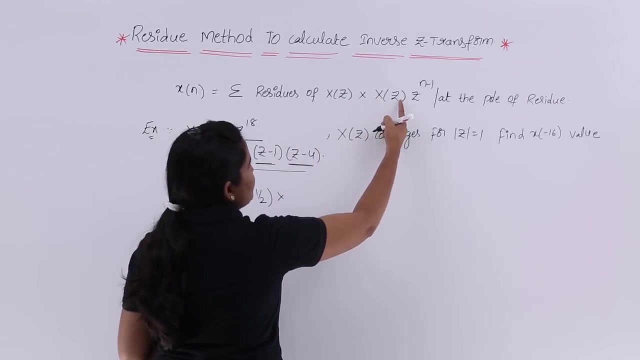 write inverse z. transform So x of n is equivalent to residue of x of z. first residue is z minus 1 by 2, z minus 1 by 2 into h of x of z. residue of x of z into x of z. x of z means this is: 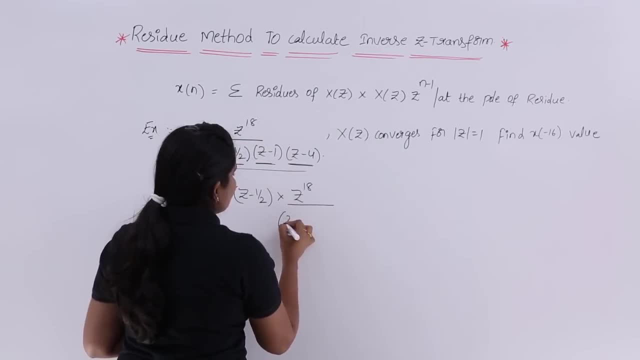 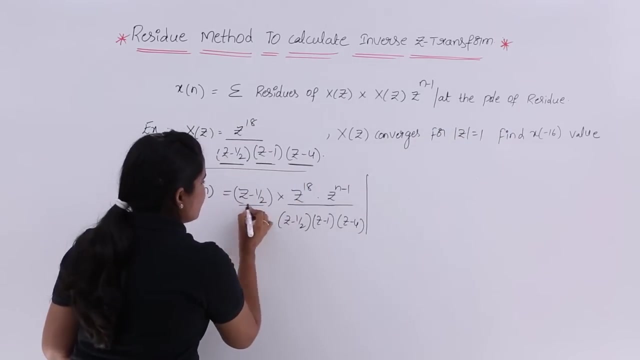 x of z z power 18 into z minus 1 by 2 z minus 1 and z minus 4 into z power n minus 1.. So this is one residue at at the pole of residue. the pole of residue is z minus 1 by. 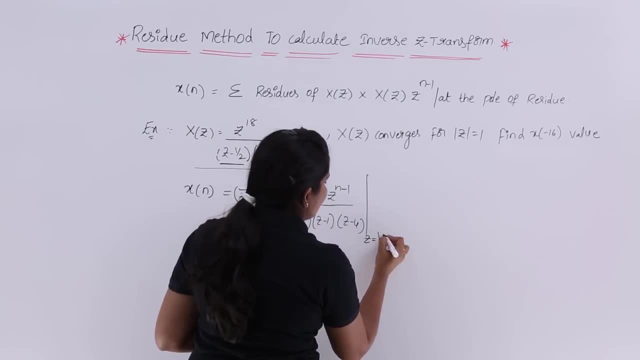 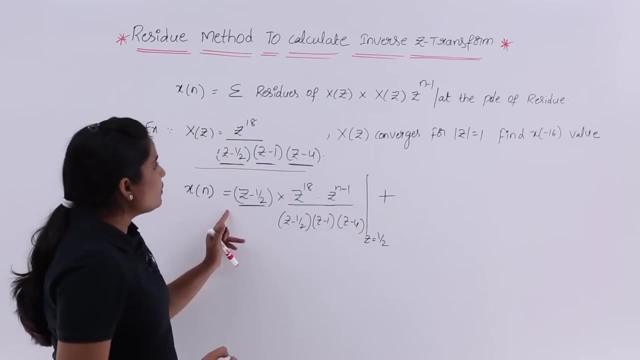 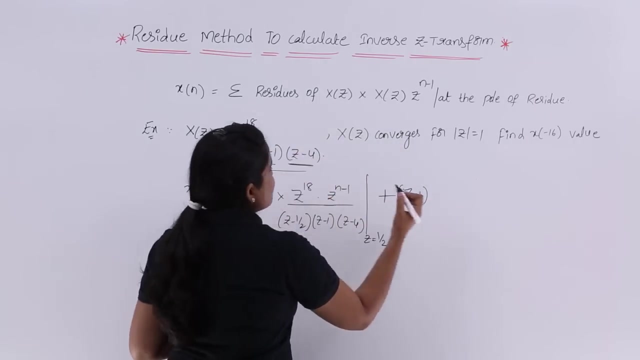 2, the pole value is 1 by 2, at z is equivalent to 1 by 2.. Now, similarly so. here we can write like this: plus. So here this second residue is z minus 1. z minus 1 into x of z means again. 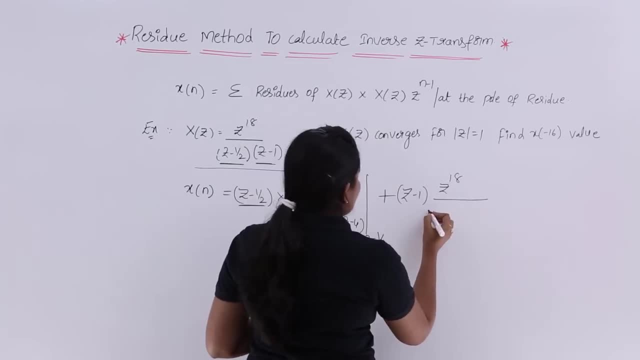 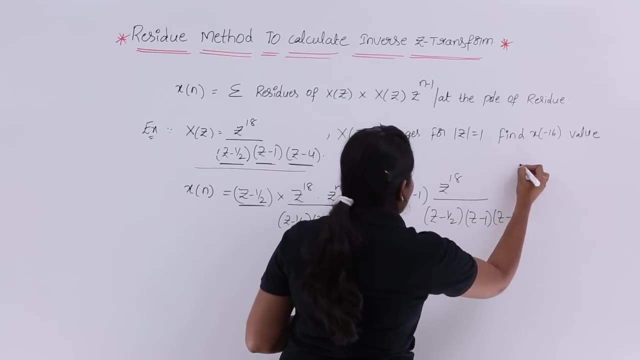 z power 18 divided by 2 raise to n. So here z minus 1 by 2, z minus 1 and z minus 4 at the pole z. power n minus 1. do not forget to write z power n minus 1 at the pole z is equivalent to 1.. In the same way, third residue: 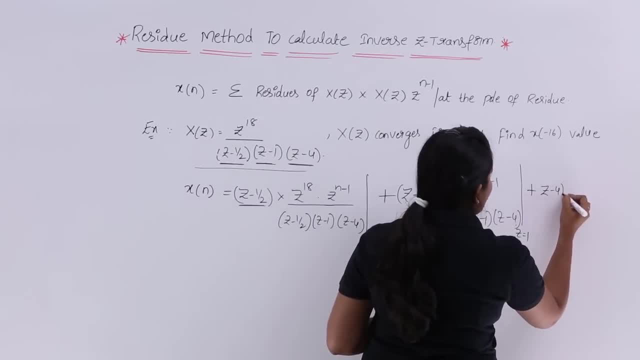 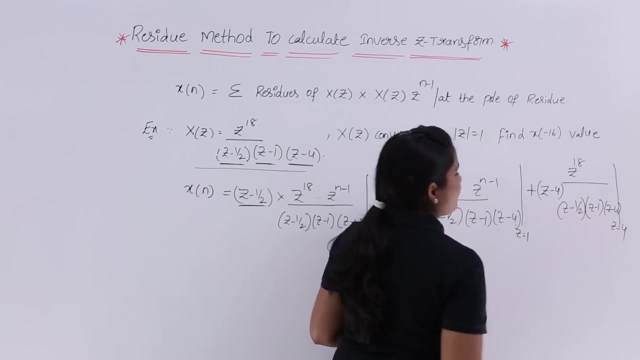 is z minus 4, residue of x of z. third, residue of x of z into x of z is z power 18 by z. power z minus 1 by 2, z minus 1, z minus 4 at z is equivalent to 4.. 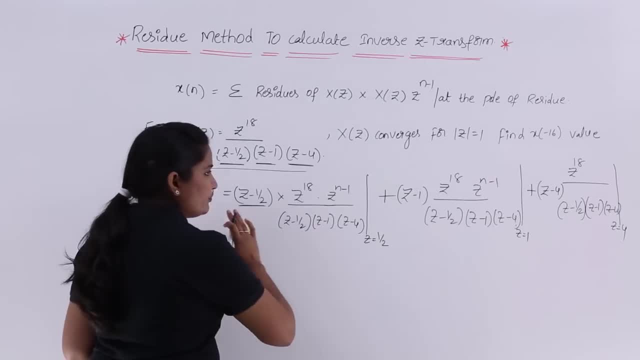 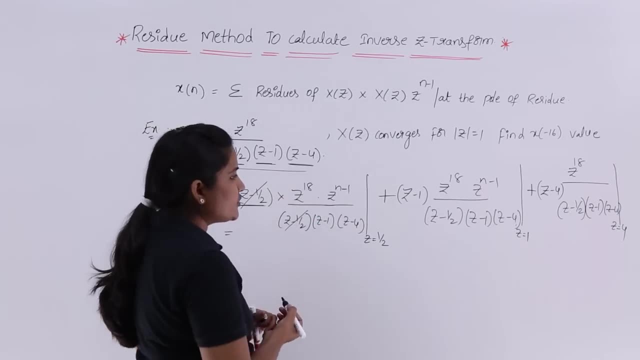 So now this is the residue theorem we are having, So we consider everything here. So now here this is equivalent to z minus 1 by 2: z minus 1 by 2 is going to cancel. z minus 1. z minus 1 is going to cancel. z minus 4, z minus 4 is going to cancel. So here z power. 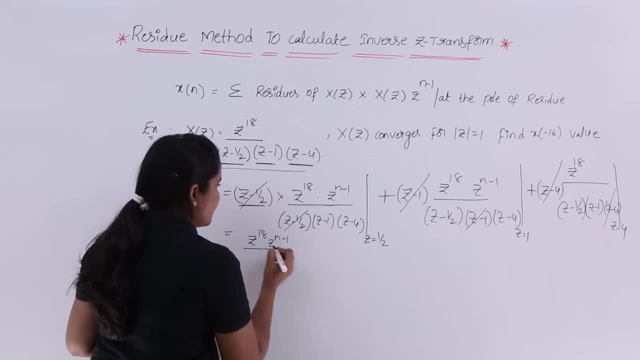 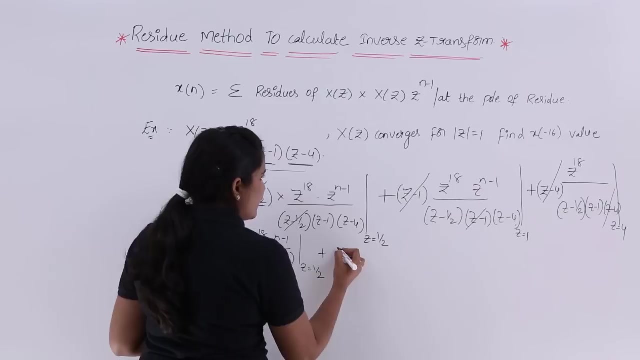 18. So z power 18 into z power n minus 1, divided by z minus 1 into z minus 4 at z is equivalent to 1 by 2. z minus 1 and z minus 4 at z is equivalent to 1 by 2. this is 1 and another. 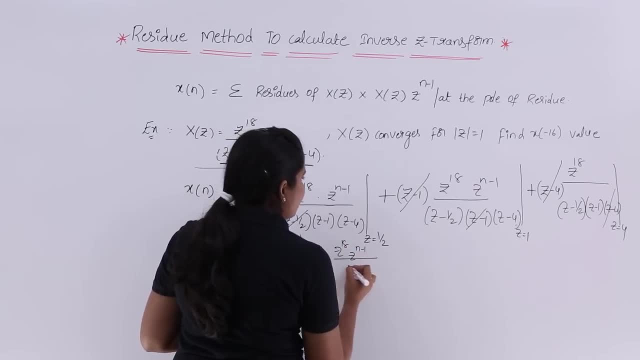 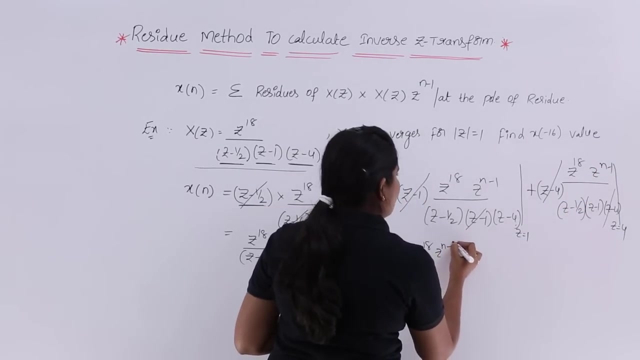 one is z power 18. z power n minus 1 divided by z minus 1, by 2, z minus 4 at z is equivalent to 1. power 18: here we forgotten to write z power n minus 1, z power n minus 1 divided by z. 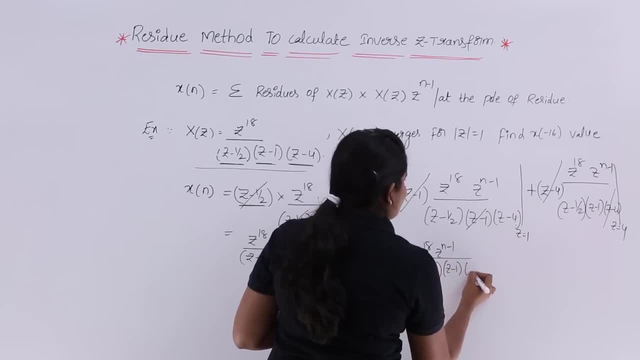 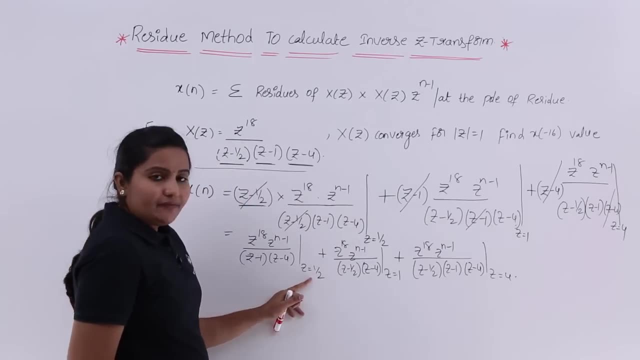 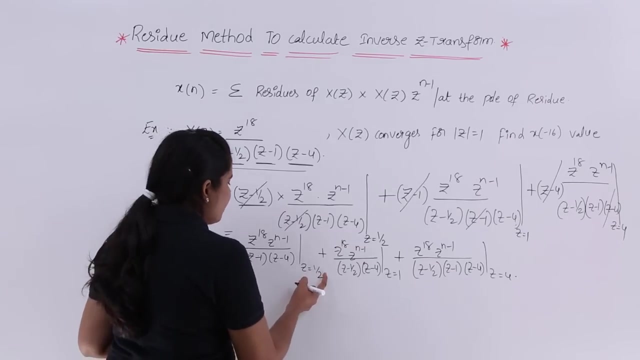 minus 1 by 2, z minus 1, z minus 4 at z is equivalent to 4.. You can see, if you consider z is equivalent to 1 by 2 here what you are going to get. So if you consider z is equivalent to 1 by 2, here you are going to get 1 by 2, whole power. 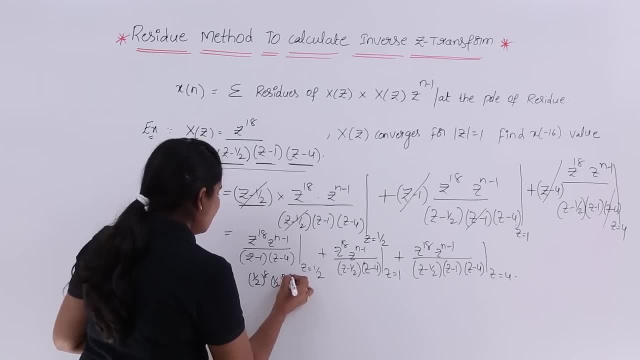 18 and 1 by 2, whole power n minus 1 divided by 1 by 2 minus 1.. So 1 by 2 minus 1 means 0.5, 0.5 into 1 by 2 minus 4.. 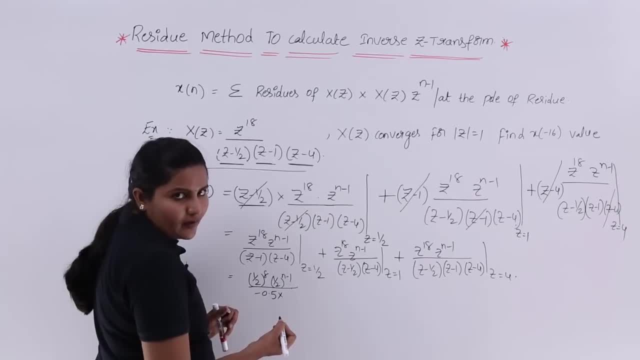 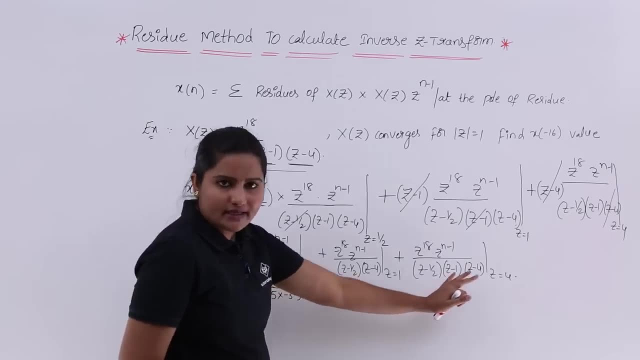 So you are getting another negative value, 3.5, you are going to get 3.5 minus 3.5, so like this. So everything you are going to get like that. So here, if you observe no need to calculate this, also, they give any condition in this. 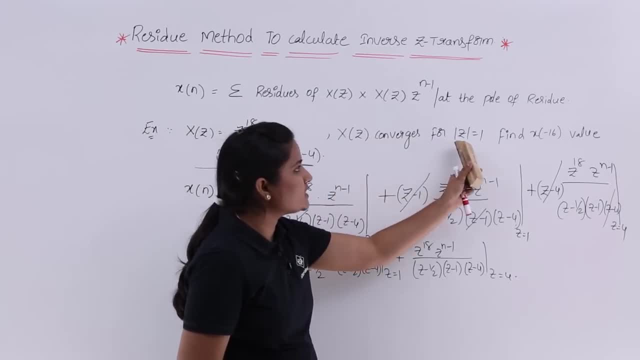 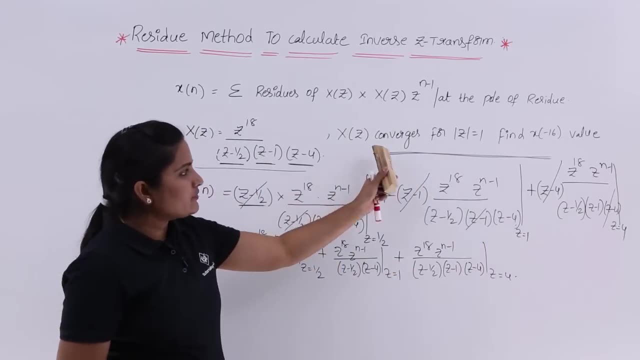 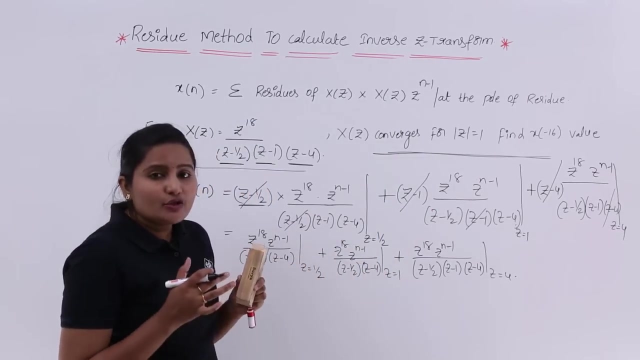 way. according to that condition you need to follow, x of z converges for mod z is equivalent to 1.. This is very, very important condition. x of z converges for mod z is equivalent to 1.. That means so here z is equivalent to plus 1 or minus 1. only you can consider all other. 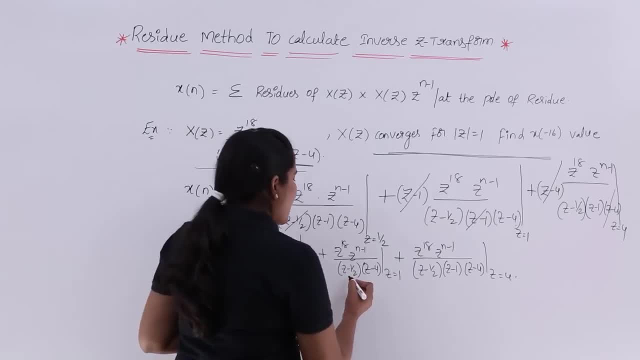 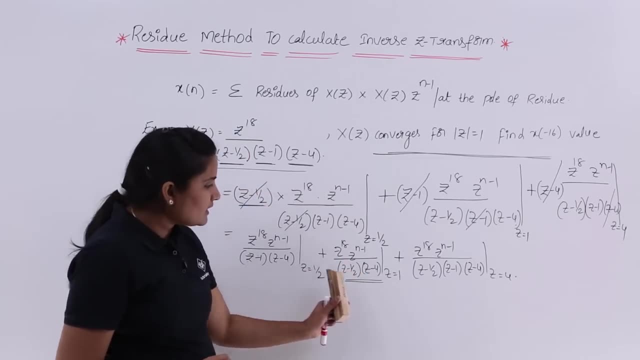 poles you are not going to consider. So here we are having a residue at z is equivalent to 1.. Only 1 residue is there At z is equivalent to 1. that residue only you need to consider as x of n. why? because 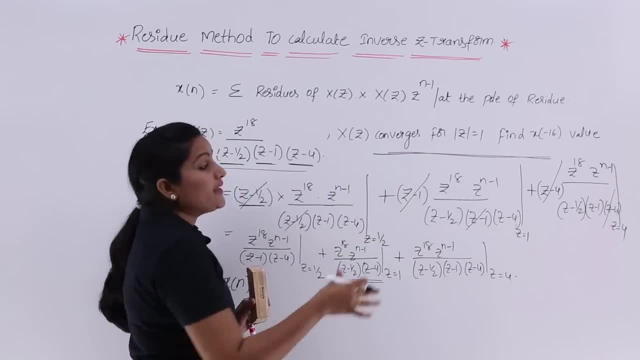 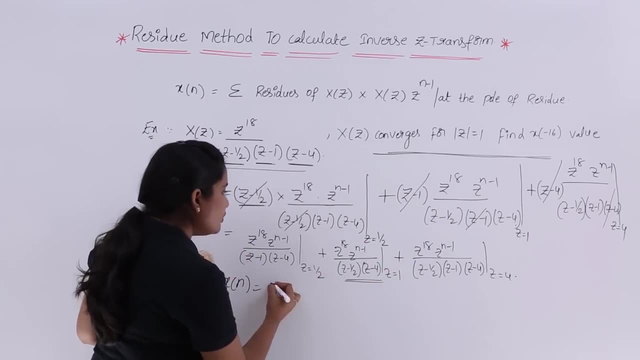 x of z converges for mod z is equivalent to 1.. If they did not, given this condition, you need to calculate everything. So x of n is equivalent to only that residue. I am considering why? because they given a specific condition: z minus 1 by 2, z minus 4, z is equivalent to 1.. 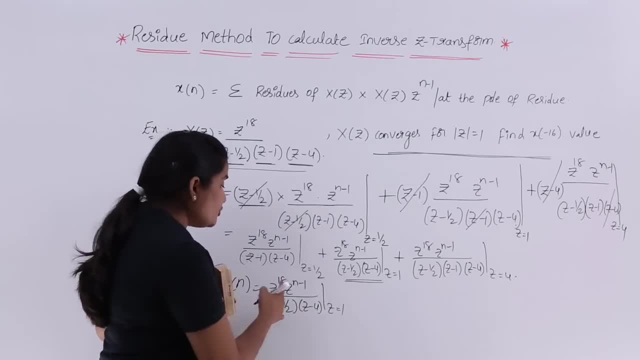 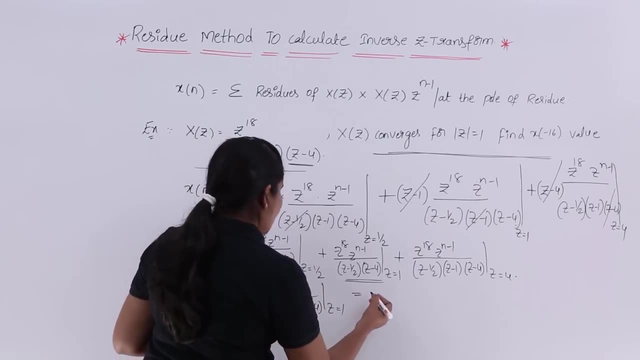 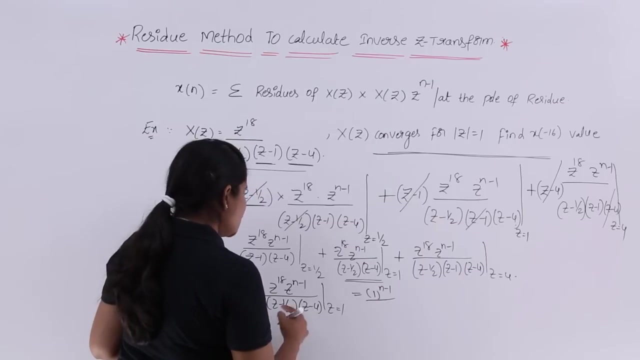 Now let us see Now, here I am substituting this one, here I am going to get 1 power 18. 1 power 18 is 1 only. So again, 1 power n minus 1. we do not know the value of this 1 power n minus 1 divided. 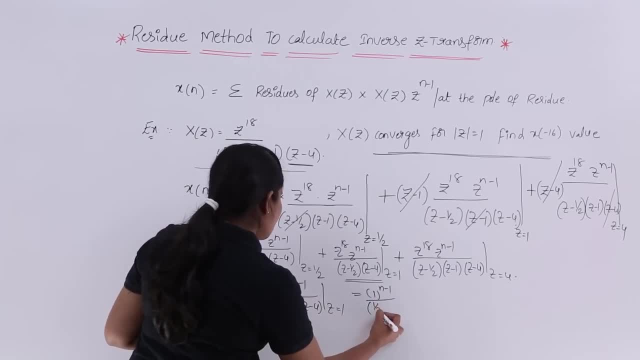 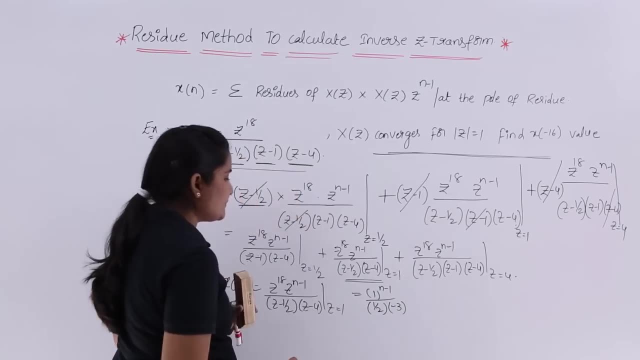 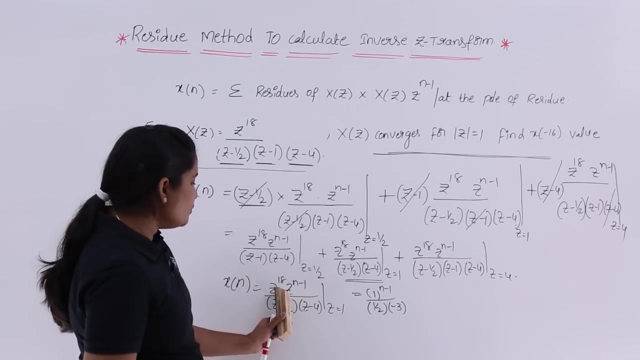 by 1 minus 1 by 2, that means 1 by 2. 1 minus 1 minus 4, that means that is equivalent to minus 3.. here I am having: x of n is equivalent to 1 power 18 into 1. power n minus 1. z minus 1 by 2 means: 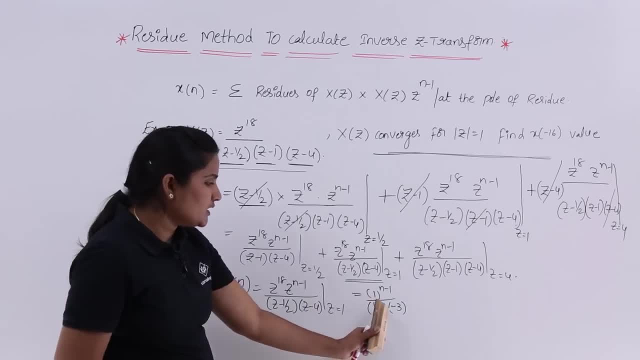 1 minus 1 by 2, and here 1 minus 4, that is equivalent to minus 3.. So now here we want x of minus 16 value. x of minus 16 value means here in place of n. if you substitute n is equivalent. 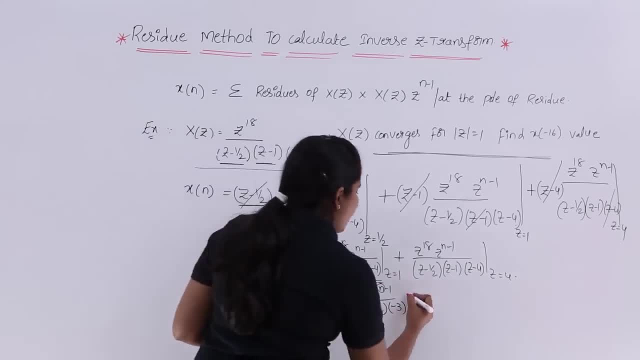 to minus 16, then you are going to get this value. that means 1 whole power minus 16, minus 1, divided by 1, by 2, into minus 3.. So now, 1 whole power minus 17. what is the value of? 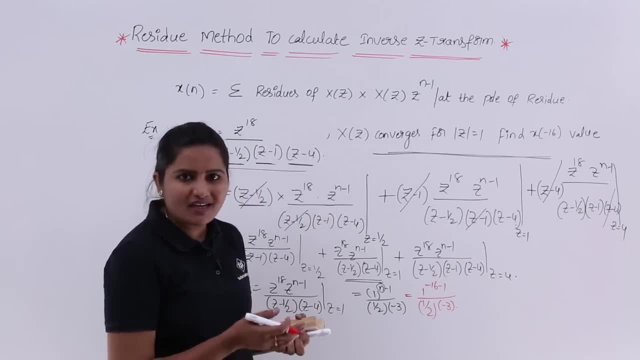 1 whole power minus 17. that is equivalent to 1, only 1 inverse is equivalent to 1, 1 whole power minus 17. you can write 1 inverse whole power 17,. 1 inverse means 1 by 1 whole. 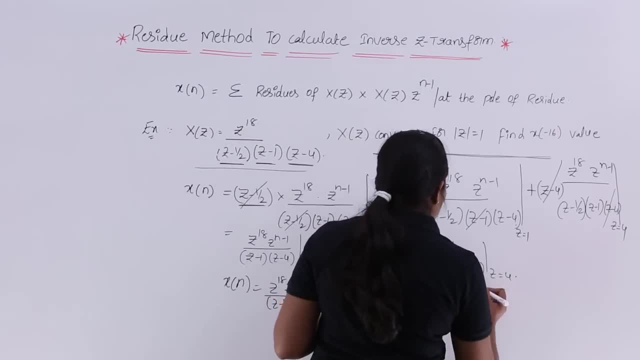 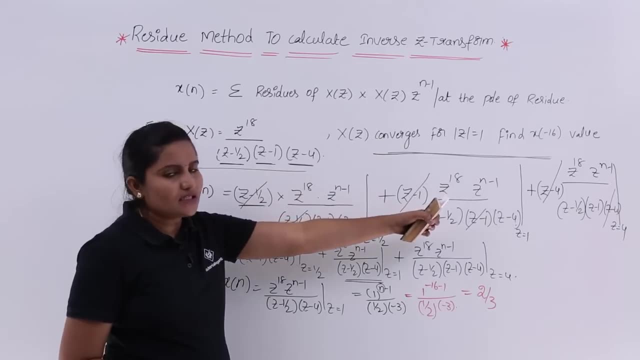 power 17.. So 1 by 1 whole power 17 is equivalent to 1.. So this is equivalent to 2 by 3. the magnitude is 2 by 3. So here the value of x of minus 16, with this transform is equivalent to 2. 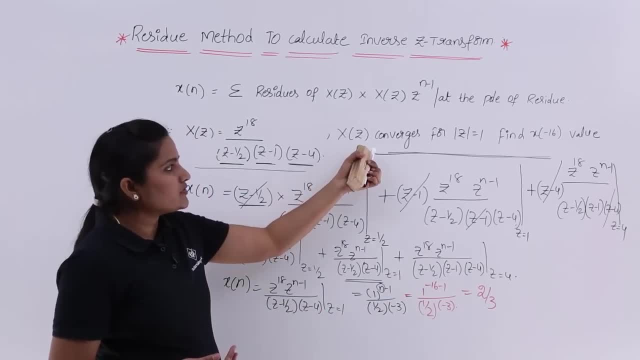 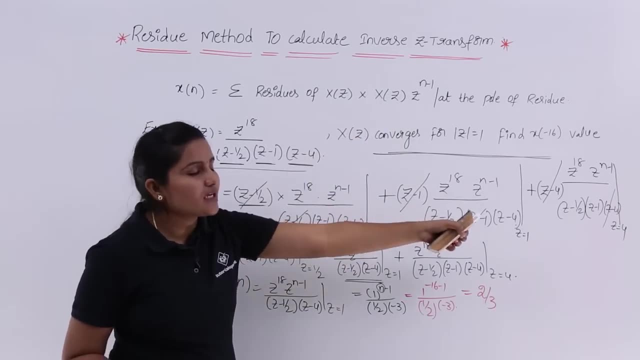 by 3.. For example, if they are saying x of z converges for mod z greater than 1.. So mod z greater than 1 means you need to consider z is equal to 4 residue value. For example, they are saying mod z: 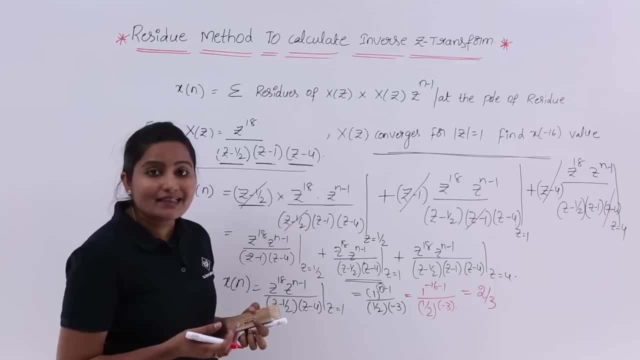 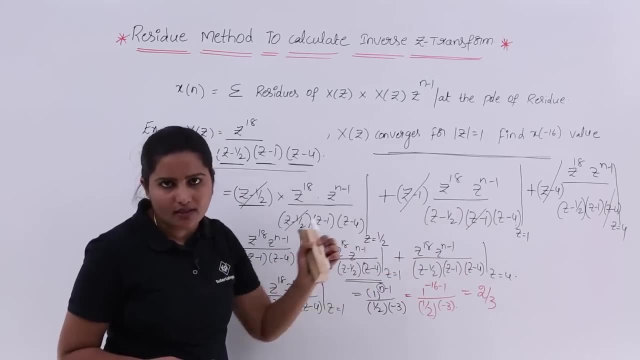 Mod z converges. for mod z converges for greater than 1 by 2.. So everything will come: 1 by 2 plus 1 plus 4.. So all this residues will come. So here they are saying only this: converges. 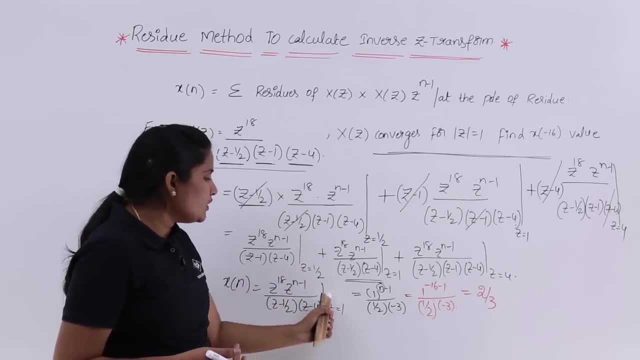 for mod z is equivalent to 1.. So that is why I consider only one value. otherwise I need to consider all the values. So, according to the ROC given in that range, how many residues are there? that many residues only you need to consider them.